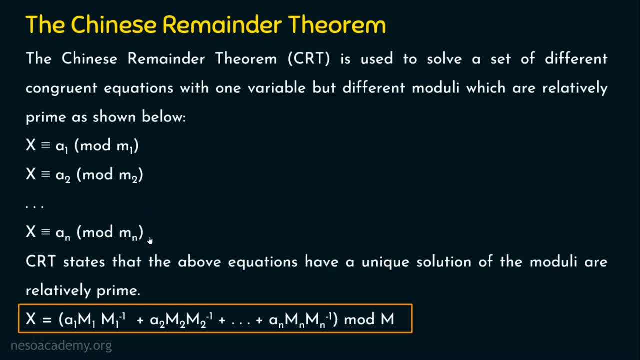 these moduli should be relatively prime. If this is the case, then we can easily find the common variable x. How, Using this formula, x is equal to a1- capital m1- capital m1, inverse, plus a2- capital m2- capital m2. 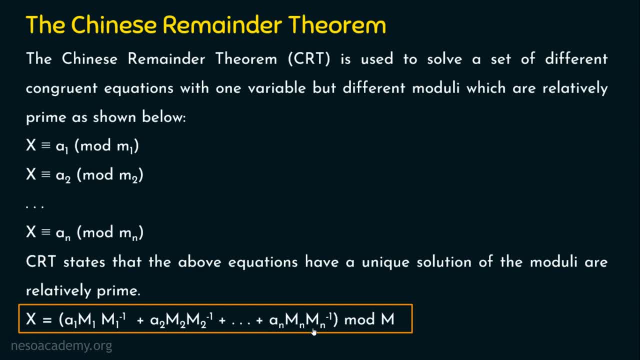 inverse up to plus an capital mn. capital mn inverse mod capital m. If we have three equations, we will take three parts. If we have four equations, we will take four parts. It depends upon the question. Let's dive into example number 2 now. 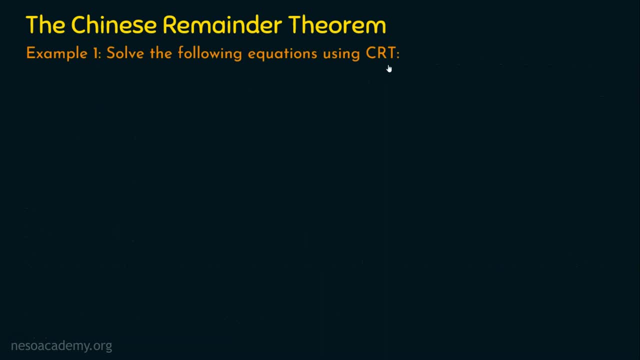 The question is: solve the following equations using Chinese remainder theorem. The equations are: 4x is congruent to 5 mod 9 and 2x is congruent to 6 mod 20.. We are required to solve these two congruent equations and we are required to find the value of x In the last example we have solved. 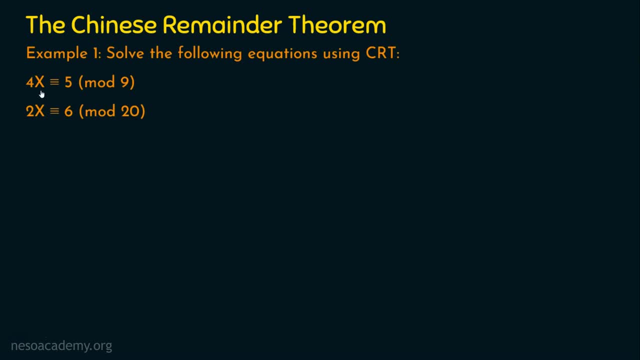 we are given with the question, which is directly x is congruent to, But here this is 4x and this is 2x. So a small trick is applied on the question here. No worries, we will break the trick first and then we will proceed with solving these. 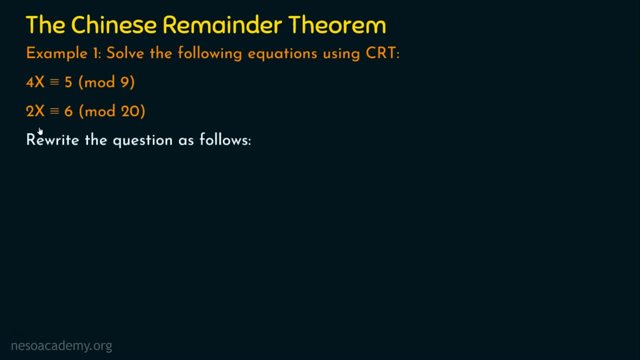 congruent equations. Let's break the trick now. So we are going to rewrite the question as follows: We have two equations, right? So I am going to take two columns. Let me place the first equation here and let me place the second equation here. So here we want to make it as x is congruent to. 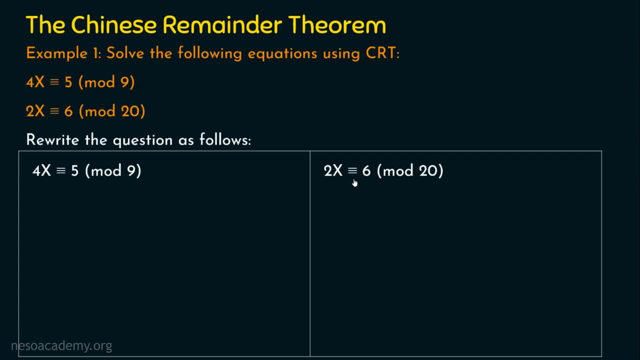 something mod 9.. Here we are going to rewrite it as x is congruent to something mod 20.. So, if you What we need to do, We need to multiply by 4 inverse, right? Is it okay to multiply 4 inverse? 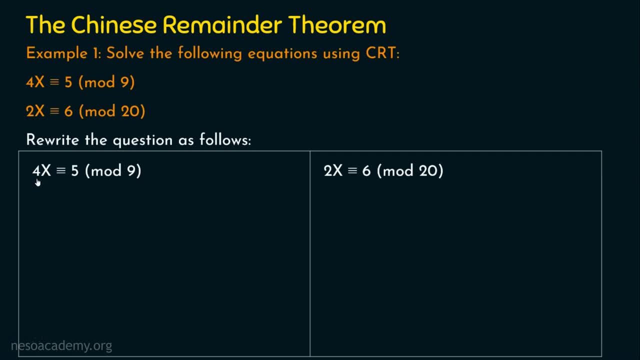 only on one side. No, that will affect the equation. So we are going to multiply 4 inverse on both the sides. So when we multiply by 4 inverse on both the sides, we get the equation as this side: 4 inverse into 4x, which is this. Then 4 inverse multiplied by 5, which is this. 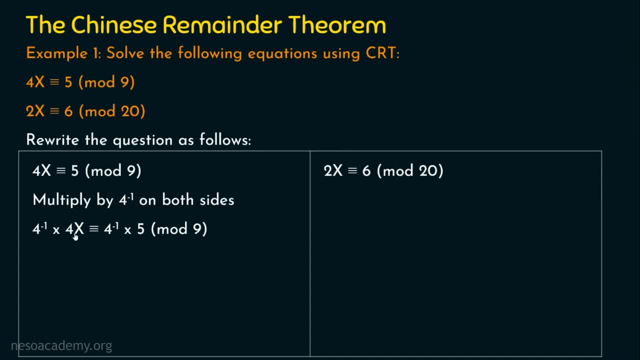 mod 9.. So 4 inverse into 4, obviously it gets nullified. we get x Here. we need to solve this 4 inverse. So, as mentioned, this side, we get x this side. we have 4 inverse into 5 mod 9.. So we are required to find what is 4 inverse mod 9, because this mod 9 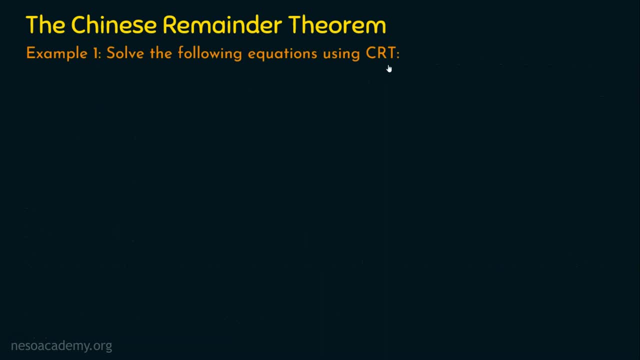 The question is: solve the following equations using Chinese remainder theorem. The equations are: 4x is congruent to 5 mod 9 and 2x is congruent to 6 mod 20.. We are required to solve these two congruent equations and we are required to find the value of x In the last example we have solved. 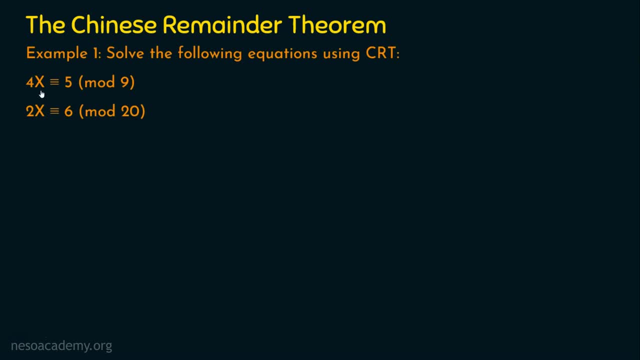 we are given with the question, which is directly x is congruent to, But here this is 4x and this is 2x. So a small trick is applied on the question here. No worries, we will break the trick first and then we will proceed with solving these. 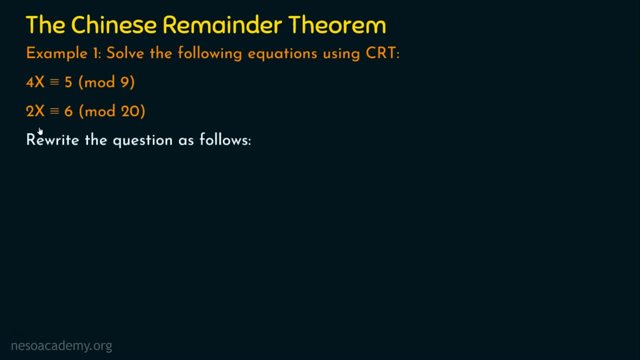 congruent equations. Let's break the trick now. So we are going to rewrite the question as follows: We have two equations, right? So I am going to take two columns. Let me place the first equation here and let me place the second equation here. So here we want to make it as x is congruent to. 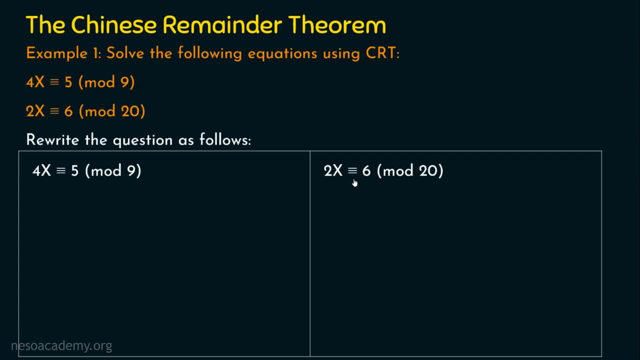 something mod 9.. Here we are going to rewrite it as x is congruent to something mod 20.. So, if you What we need to do, We need to multiply by 4 inverse, right? Is it okay to multiply 4 inverse? 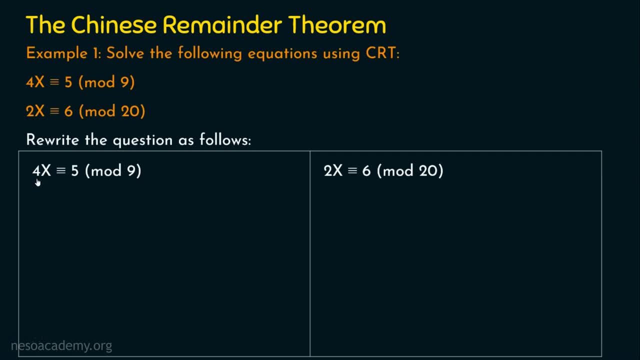 only on one side. No, that will affect the equation. So we are going to multiply 4 inverse on both the sides. So when we multiply by 4 inverse on both the sides, we get the equation as this side: 4 inverse into 4x, which is this. Then 4 inverse multiplied by 5, which is this. 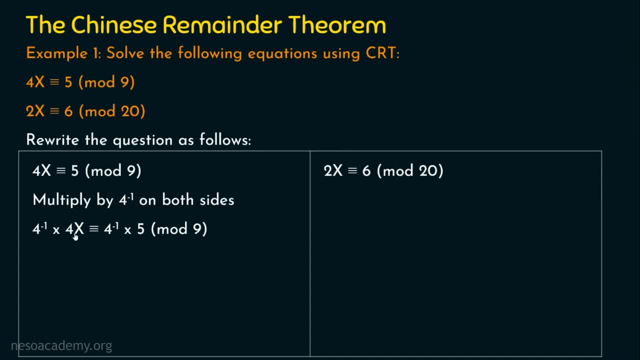 mod 9.. So 4 inverse into 4, obviously it gets nullified. we get x Here. we need to solve this 4 inverse. So, as mentioned, this side, we get x this side. we have 4 inverse into 5 mod 9.. So we are required to find what is 4 inverse mod 9, because this mod 9 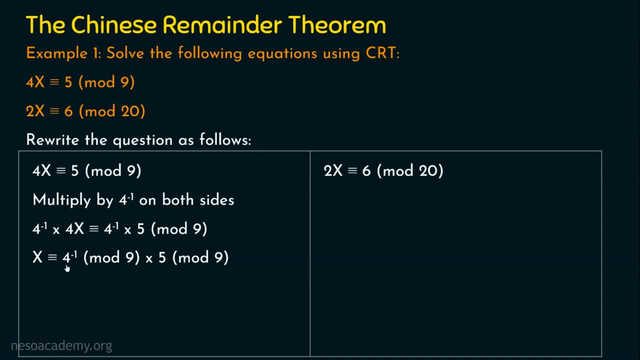 is applicable for 4 inverse as well. So we are going to find the multiplicative inverse of 4 mod 9.. We will start applying with 1.. 4 into 1 is 4.. 4 mod 9 is 4, not 1, because when a multiplicative 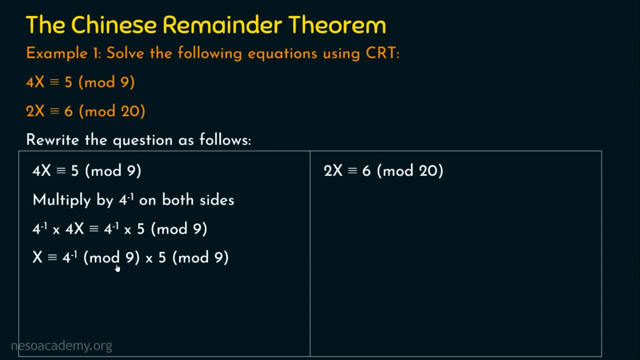 inverse. when it is multiplied with that number, we should get 1 as the remainder. But in this case 1 is not the multiplicative inverse. Let's try with 2.. 2 into 4 is 8.. When 8 is divided by 9, we get 8 as the remainder, not 1.. Let's try 3.. 4 into 3 is 12.. 12 mod. 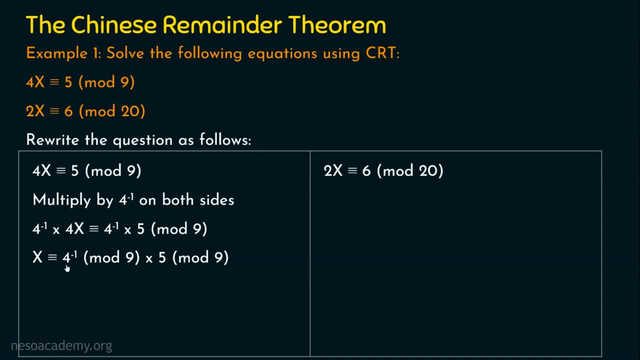 is applicable for 4 inverse as well. So we are going to find the multiplicative inverse of 4 mod 9.. We will start applying with 1.. 4 into 1 is 4.. 4 mod 9 is 4, not 1, because when a multiplicative 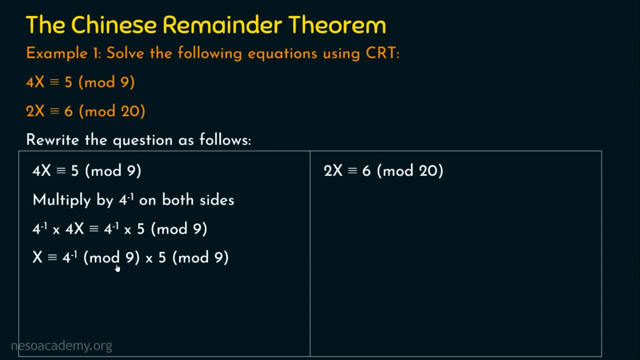 inverse. when it is multiplied with that number, we should get 1 as the remainder. But in this case 1 is not the multiplicative inverse. Let's try with 2.. 2 into 4 is 8.. When 8 is divided by 9, we get 8 as the remainder, not 1.. Let's try 3.. 4 into 3 is 12.. 12 mod. 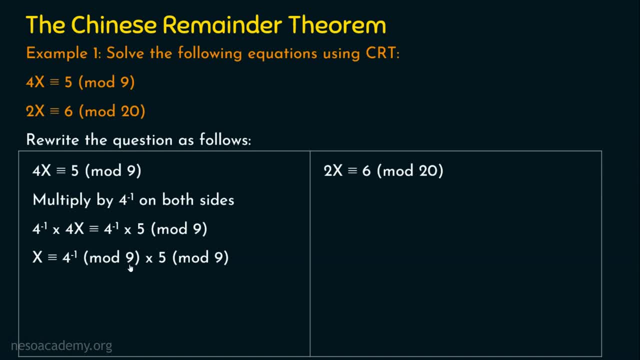 9 is 3.. Let's try 4.. 4 into 4 is 16.. 16 mod 9, we get 7.. Let's try 5.. 4 into 5 is 20.. 20 mod 9, we get 2.. Let's try 6.. 6 into 4 is 24.. 24 mod 9.. 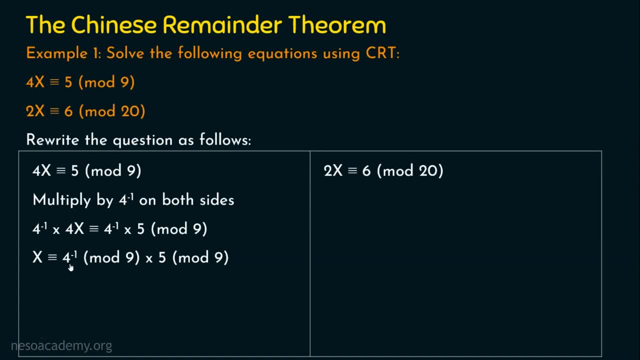 What we will get. We get 6, right, So let's try 7.. 4 into 7 is 28.. 28, when it is divided by 9, we get 1 as the remainder. So we are going to find the multiplicative inverse of 4 mod 9.. 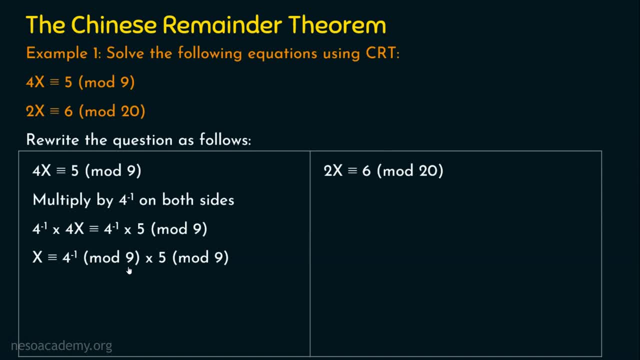 You can manually try this or you can refer my previous lecture to find out the multiplicative inverse. using extended Euclidean algorithm. 7 is the multiplicative inverse of 4.. So 4 into 7 is 28.. 28 mod 9.. 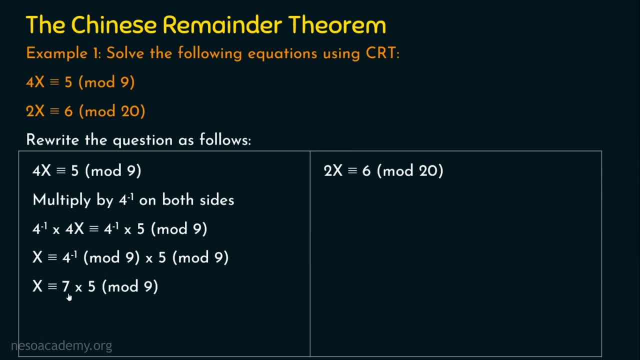 28, when it is divided by 9, we get 1 as the remainder. So 7 is the multiplicative inverse of 4 mod 9.. Then we have this 5 mod 9 here I am just retaining this. here We get 7 into. 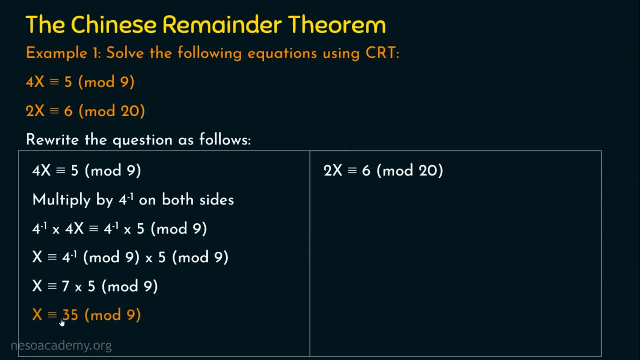 5 mod 9.. What is 7 into 5?? It is 35. So 35 mod 9 is the answer. If you want, you can still reduce this right 35. when it is divided by 9, we get 8 as the remainder You can take. 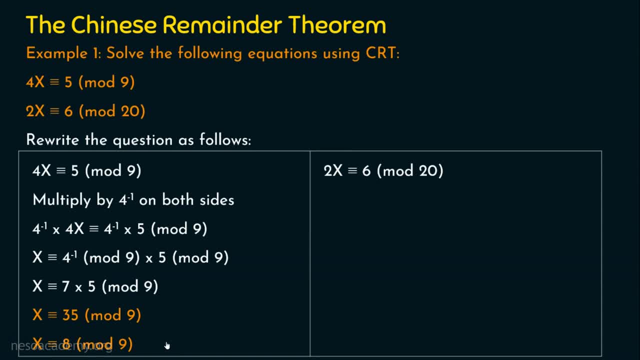 either this or this. I always recommend you to go for smaller numbers. So 35 mod 9 is 8 mod 9.. Just divide 35 by 9.. 9 3 times 27 and the remainder is 8.. So we are reducing this as. 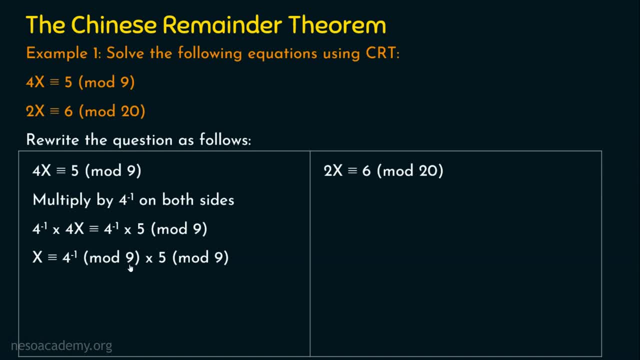 9 is 3.. Let's try 4.. 4 into 4 is 16.. 16 mod 9, we get 7.. Let's try 5.. 4 into 5 is 20.. 20 mod 9, we get 2.. Let's try 6.. 6 into 4 is 24.. 24 mod 9.. 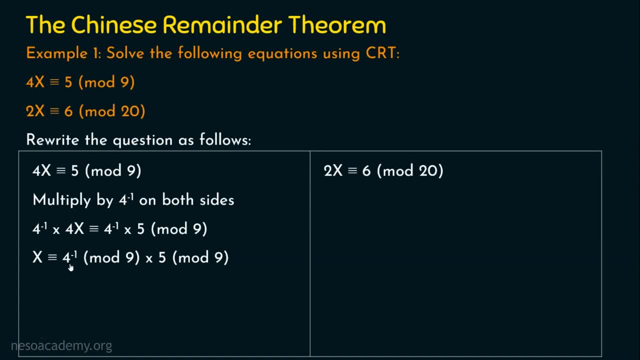 What we will get. We get 6, right, So let's try 7.. 4 into 7 is 28.. 28, when it is divided by 9, we get 1 as the remainder. So we are going to find the multiplicative inverse of 4 mod 9.. 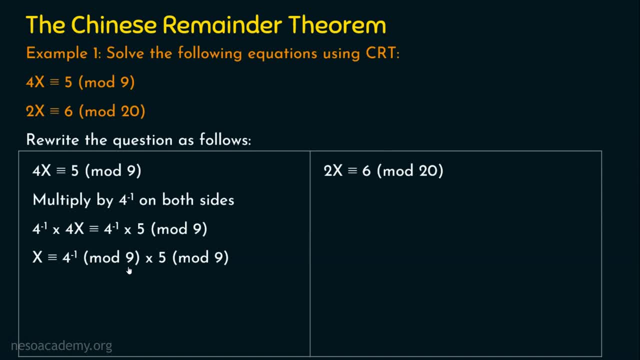 You can manually try this or you can refer my previous lecture to find out the multiplicative inverse. using extended Euclidean algorithm. 7 is the multiplicative inverse of 4.. So 4 into 7 is 28.. 28 mod 9.. 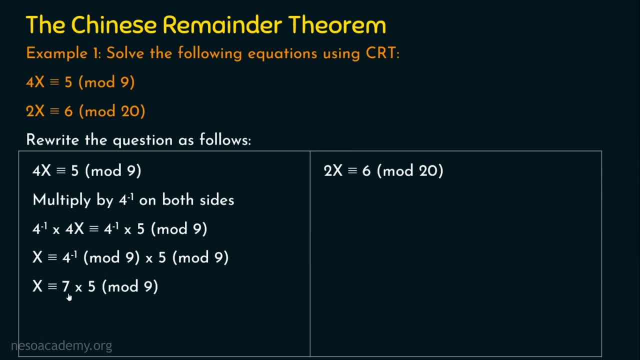 28, when it is divided by 9, we get 1 as the remainder. So 7 is the multiplicative inverse of 4 mod 9.. Then we have this 5 mod 9 here I am just retaining this. here We get 7 into. 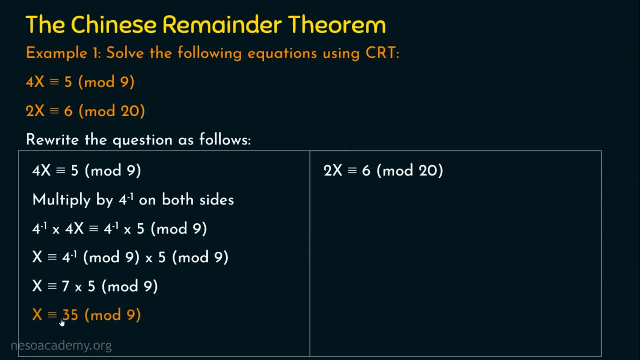 5 mod 9.. What is 7 into 5?? It is 35. So 35 mod 9 is the answer. If you want, you can still reduce this right 35. when it is divided by 9, we get 8 as the remainder You can take. 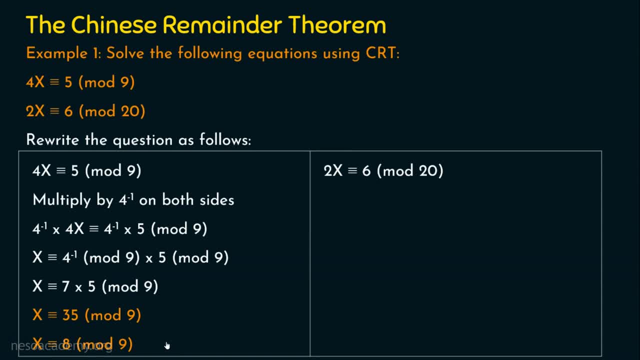 either this or this. I always recommend you to go for smaller numbers. So 35 mod 9 is 8 mod 9.. Just divide 35 by 9.. 9, 3 times 27 and the remainder is 8.. So we are reducing this as. 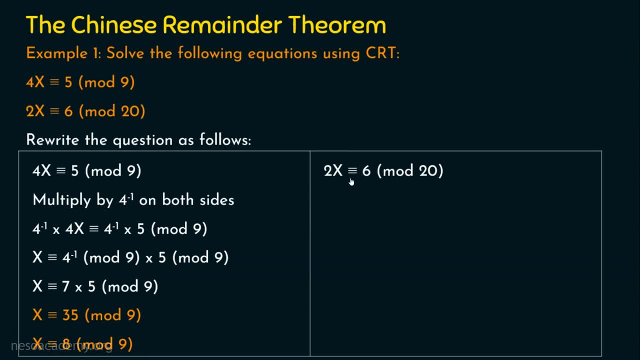 x is congruent to 8 mod 9. But this side is so simple. Why? Because here we have 2. Here also we have a number that can be divisible by 2. So we can rewrite the 6 as 2 into 3, right So? 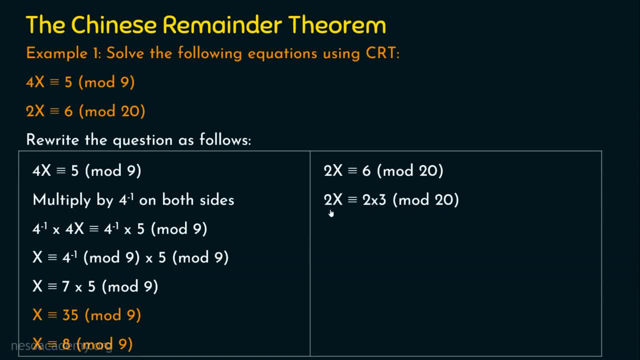 2x is congruent to 2 into 3 mod 20.. When we divide by 2 on both the sides, we get x is congruent to 3 mod 20.. So we get 8 mod 9.. So we are reducing this as x is congruent to 8 mod 9.. But this side. 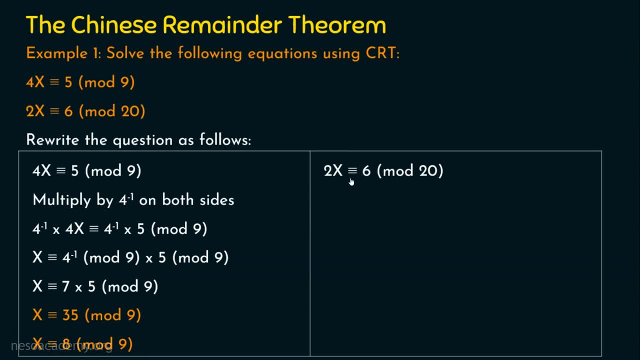 x is congruent to 8 mod 9. But this side is so simple. Why? Because here we have 2. Here also we have a number that can be divisible by 2. So we can rewrite the 6 as 2 into 3, right So? 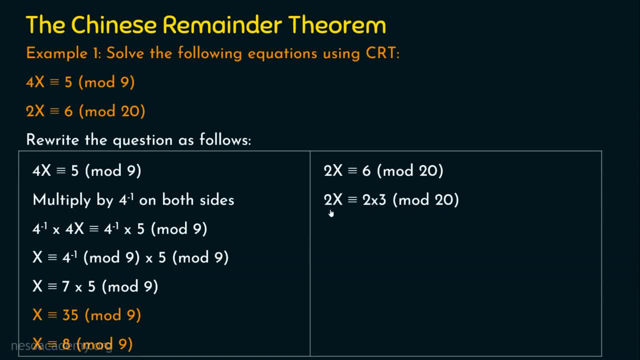 2x is congruent to 2 into 3 mod 20.. When we divide by 2 on both the sides, we get x is congruent to 3 mod 20.. So we get 8 mod 9.. So we are reducing this as x is congruent to 8 mod 9.. But this side. 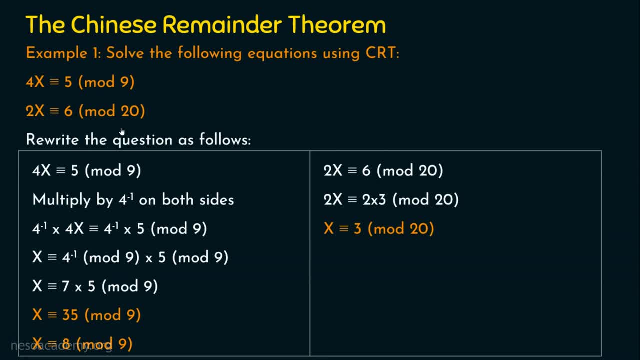 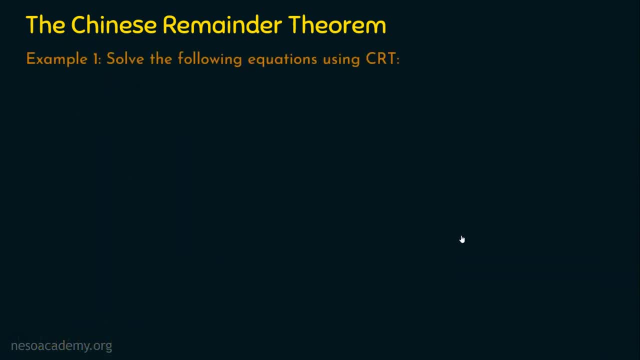 we got the equations now, So these 2 equations can be rewritten as x is congruent to 8 mod 9 and x is congruent to 3 mod 20.. Let's solve this question using these 2 congruent equations. 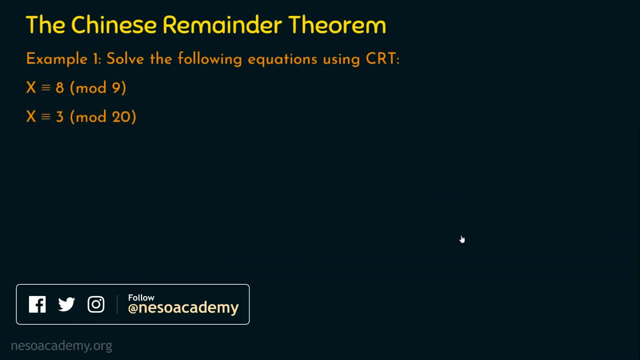 Now we have simplified the question. in the format, x is congruent to a1 mod m1 and x is congruent to a2 mod m2.. Please note: here we have only 2 different congruent equations. Let's solve this question now In order to find the value of x. we note the formula is: 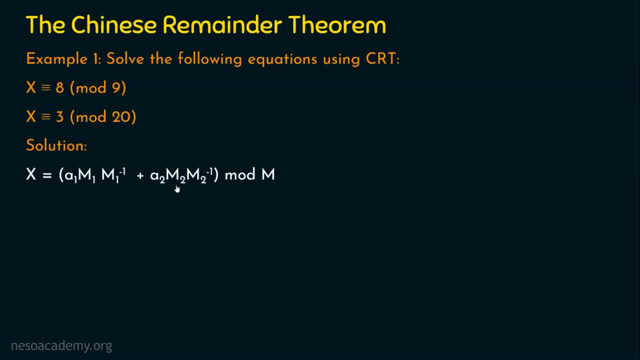 equal to a1 capital m1 capital m1 inverse, plus a2 capital m2 capital m2 inverse. That's it Why I'm stopping up to 2? Because we have 2 equations Mod m. Now what are all the given data We can? 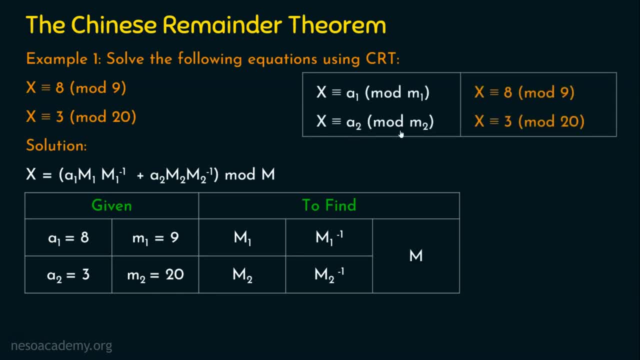 easily find the given data. We have only 2 congruent equations, So I'm just comparing the equation with the question. So what's the given data? a1 is 8 and a2 is 3. So a1 is equal. 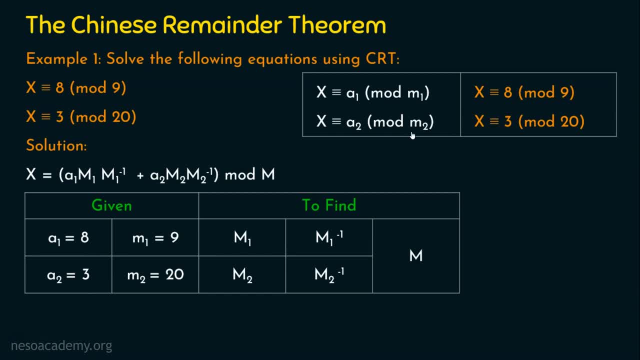 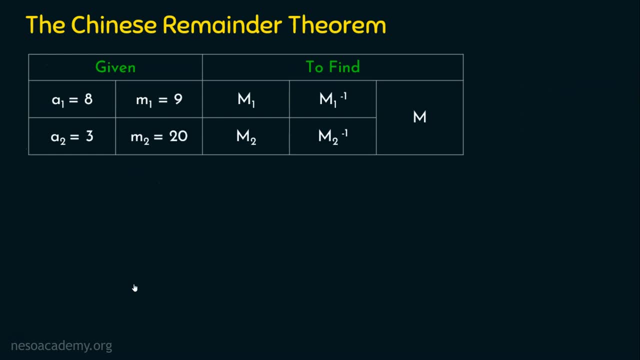 to 8 and a2 is equal to 3. And small m1 is 9 and small m2 is 20.. So 9 and 20 are placed in the places m1 and m2 respectively. Let's solve this question by. 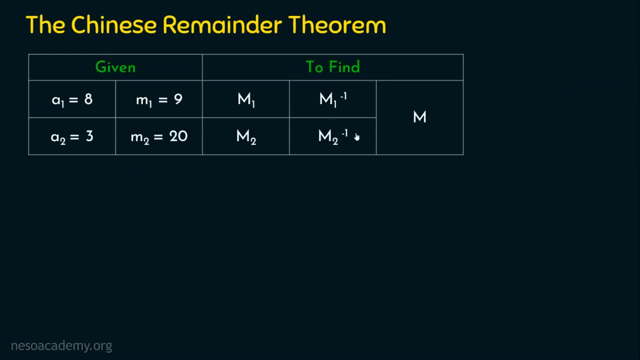 finding out capital m1, capital m2, their corresponding inverses and then capital m. Firstly, let's focus on finding the capital m value. We know capital m is the product of small m1 and small m2.. So m is equal to m1 into m2.. Please note: these are small m, So when you apply, 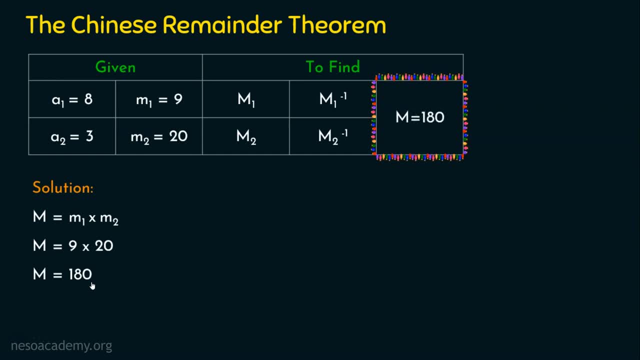 capital m into m2, capital m is equal to m, So we found out the value of capital m, which is 180.. Let's now move on to finding capital m1 and capital m2.. We know how to find this: Capital m1 is equal. 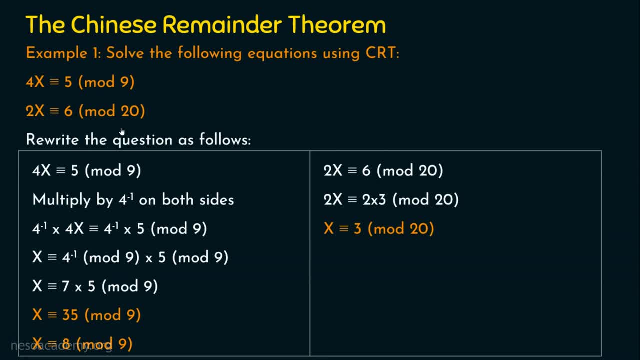 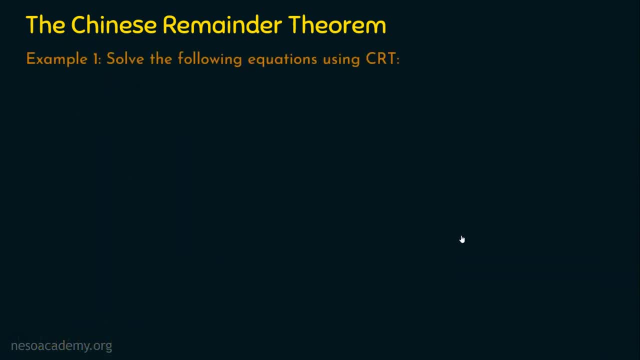 we got the equations now, So these 2 equations can be rewritten as x is congruent to 8 mod 9 and x is congruent to 3 mod 20.. Let's solve this question using these 2 congruent equations. 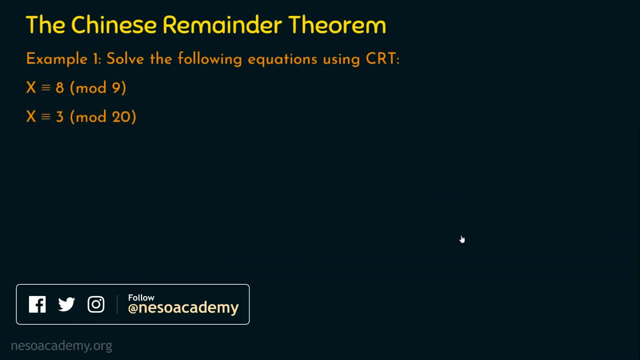 Now we have simplified the question. in the format, x is congruent to a1 mod m1 and x is congruent to a2 mod m2.. Please note: here we have only 2 different congruent equations. Let's solve this question now In order to find the value of x. we note the formula is: 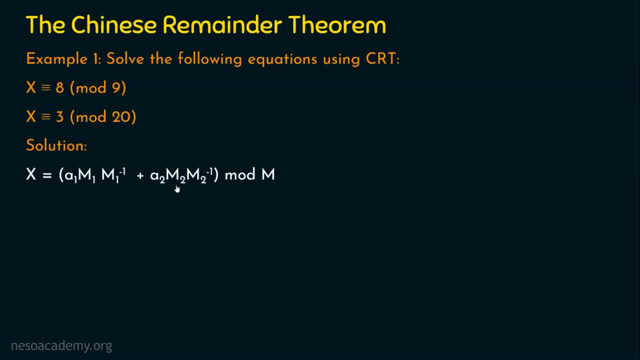 equal to a1 capital m1 capital m1 inverse, plus a2 capital m2 capital m2 inverse. That's it Why I'm stopping up to 2? Because we have 2 equations Mod m. Now what are all the given data We can? 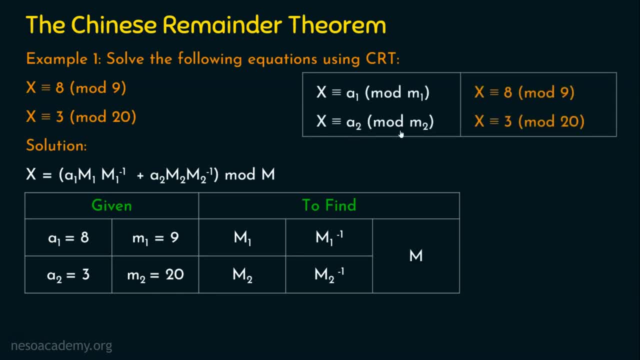 easily find the given data. We have only 2 congruent equations, So I'm just comparing the equation with the question. So what's the given data? a1 is 8 and a2 is 3. So a1 is equal. 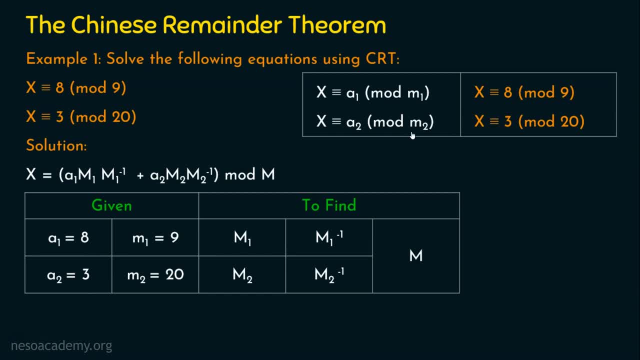 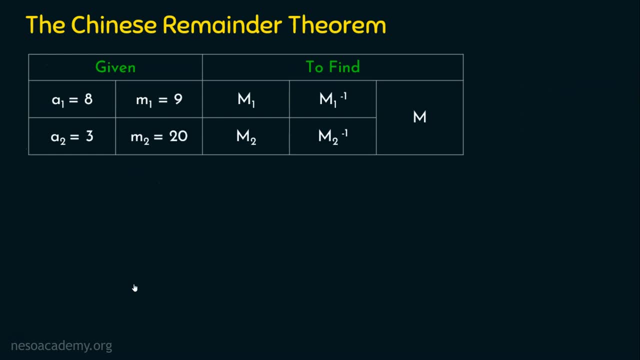 to 8 and a2 is equal to 3. And small m1 is 9 and small m2 is 20.. So 9 and 20 are placed in the places m1 and m2 respectively. Let's solve this question by. 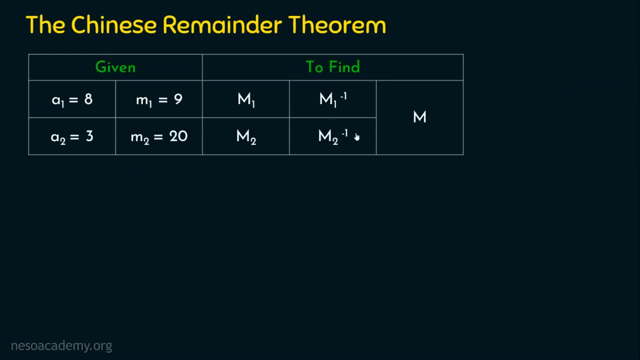 finding out capital m1, capital m2, their corresponding inverses and then capital m. Firstly, let's focus on finding the capital m value. We know capital m is the product of small m1 and small m2.. So m is equal to m1 into m2.. Please note: these are small m, So when you apply, 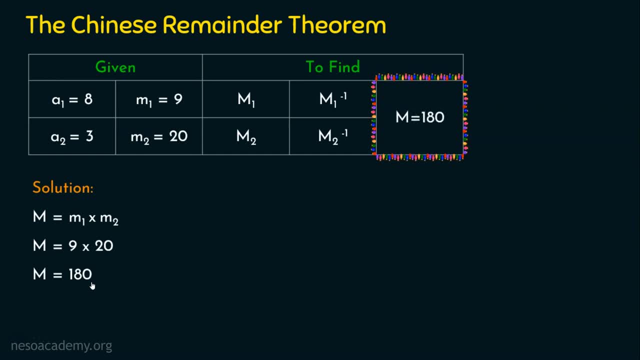 capital m into m2, capital m is equal to m2.. So we found out the value of capital m, which is 180.. Let's now move on to finding capital m1 and capital m2.. We know how to find this. Capital m1 is equal. 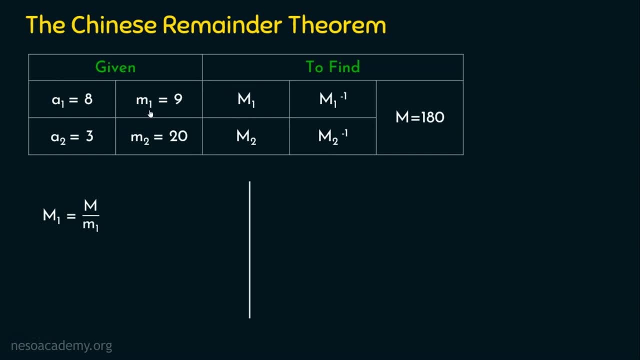 to capital m upon small m1, because we are going to find capital m1. So we need to use this value right. So capital m1 is equal to capital m upon small m1 and capital m2 is equal to capital m upon. 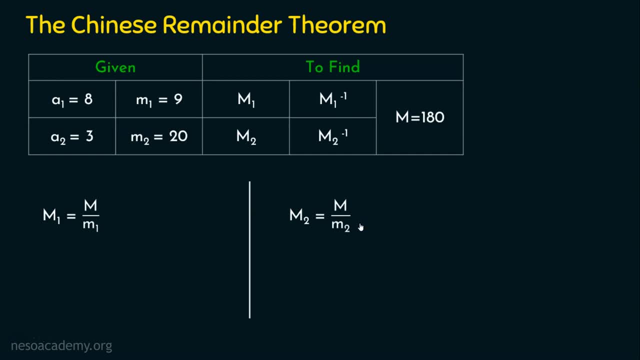 small m2.. If you are directly watching this lecture, I request you to watch my previous lecture. you will get a better insight about Chinese remainder theorem and how to solve this. So when we substitute the values, we get capital m1 is equal to 20 and capital m2 is equal to 9.. 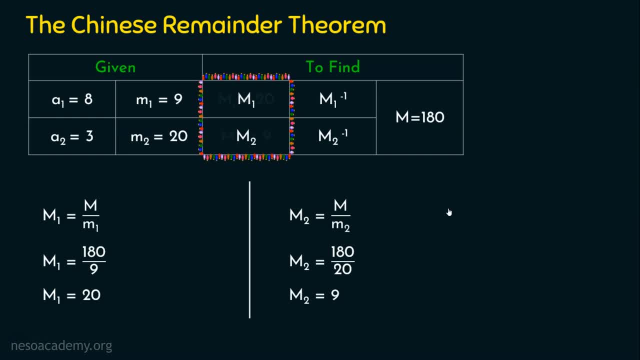 So we found out the value of capital m1 and capital m2.. I am just placing this in the table. Now the only thing that is required is to find the inverses, that is, m1 inverse and m2 inverse. 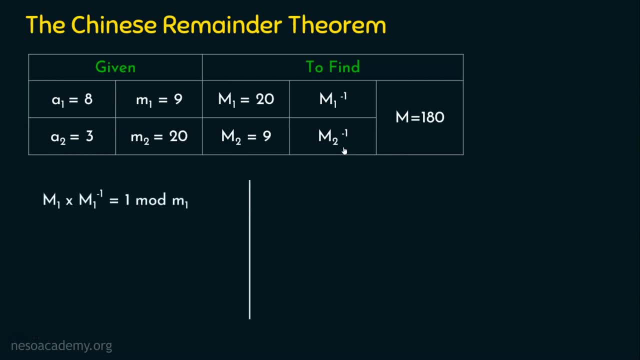 Let's find that We know how to find m1 inverse and m2 inverse. When capital m1 is multiplied by capital m1, capital m1 is equal to capital m1.. So capital m1 is equal to capital m2.. So capital m1 is. 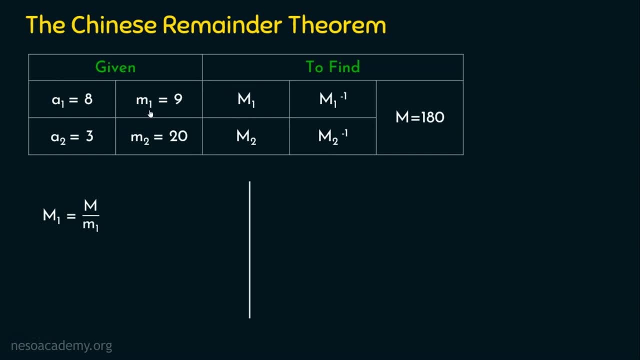 to capital m upon small m1, because we are going to find capital m1. So we need to use this value right. So capital m1 is equal to capital m upon small m1 and capital m2 is equal to capital m upon. 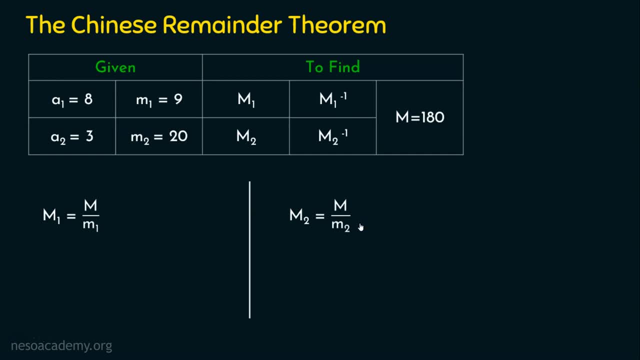 small m2.. If you are directly watching this lecture, I request you to watch my previous lecture. get a better insight about Chinese remainder theorem and how to solve this. So when we substitute the values, we get capital m1 is equal to 20 and capital m2 is equal to 9.. So we found: 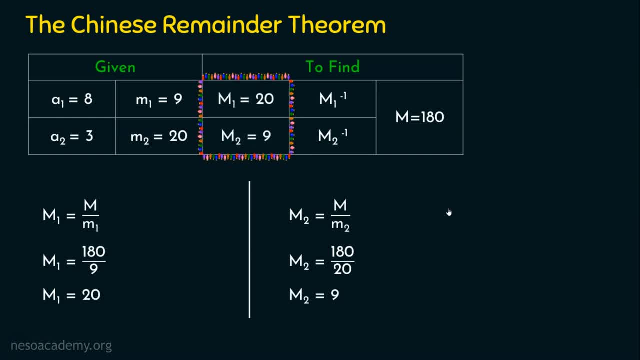 out the value of capital m1 and capital m2.. I am just placing this in the table. Now the only thing that is required is to find the inverses, That is, m1 inverse and m2 inverse. Let's find that. We know how to find m1 inverse and m2 inverse When capital m1 is multiplied by capital. 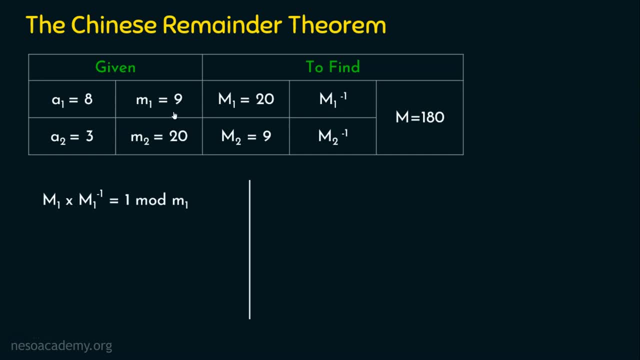 m1, capital m1 is equal to capital m1.. So we know how to find capital m1 and capital m2.. So capital m1 inverse, we get 1 as the remainder. when we do mod small m1, right, Which is this: 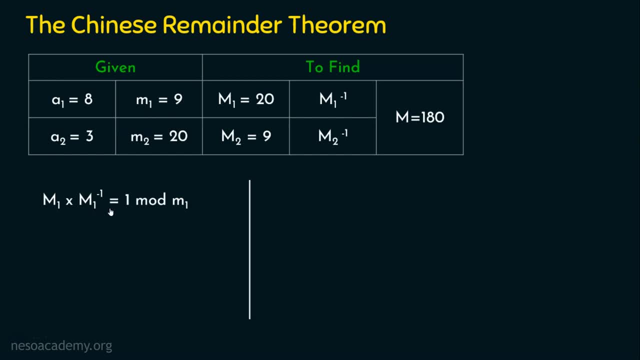 So capital m1, when it is multiplied by capital m1 inverse, we get 1 as the remainder under mod small m1. Similarly, capital m2, when it is multiplied by capital m2 inverse, we get 1 mod small m2.. We know what is the value of capital m1 and capital m2.. So firstly, 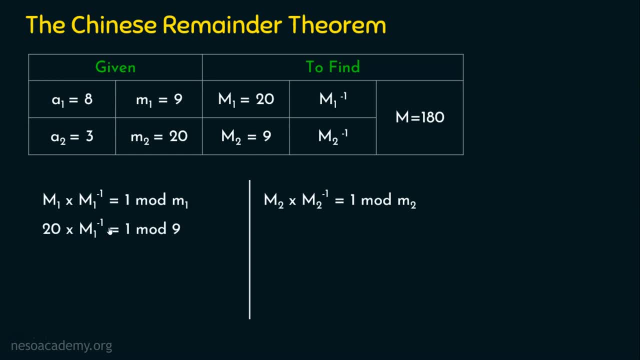 let's focus on this equation. We get 20 into capital. m1. inverse is equal to 1 mod 9, because small m1 is 9, which is this. So 20 into what we get the whole product. when it is divided by 9, we get 1 as the remainder. Let's start applying with 1.. You can also go for. 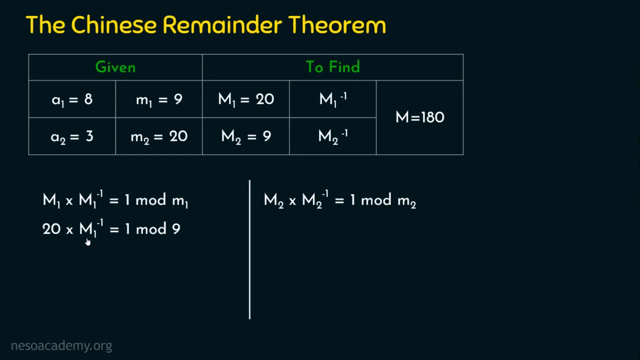 extended Euclidean algorithm to find the multiplicative inverse. Since these are all smaller numbers, I am going directly. Let's try with 1.. 20 into 1 is 20.. 20 when it is divided by 9, we get 2 as the remainder. So 1 is not the multiplicative inverse of 20 mod 9.. Let's try 2.. 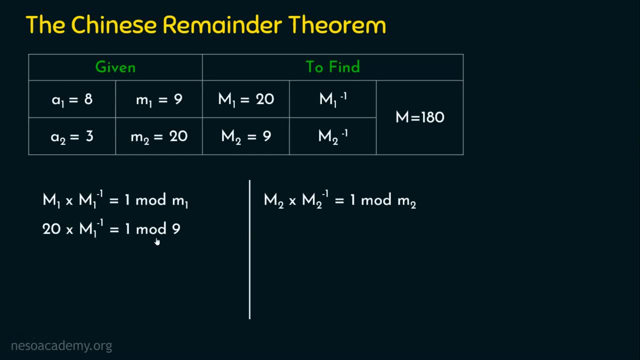 20 into 2 is 40.. No, we don't get 1 as the remainder when we divide 40 by 9.. Let's try 3.. No, Let's try 4.. No, Let's try 5.. Yes, 20 into 5 is 100.. 100 when it is divided by 9.. 9, 11 times 99. So 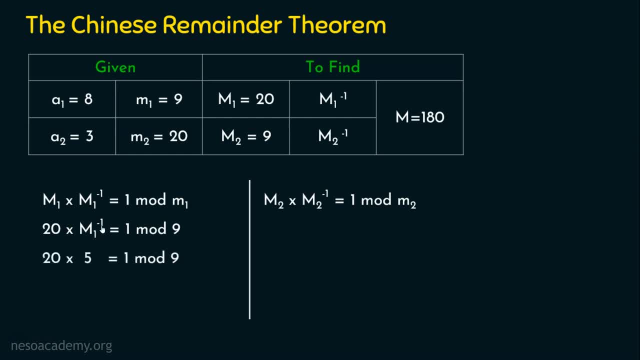 we get 1 as the remainder. So obviously, capital m1 inverse is 5.. That's what we obtained. Let's move on to the second part, which is this: We know what is the value of capital m2, which is 9.. So I am placing this 9 here. 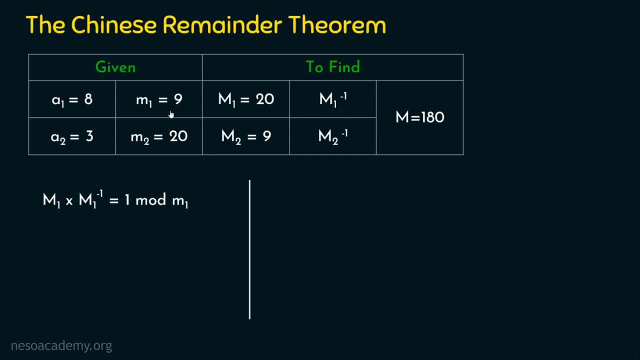 equal to capital m1 inverse, We get 1 as the remainder. when we do mod small m1, right, Which is this? So capital m1, when it is multiplied by capital m1 inverse, we get 1 as the remainder. 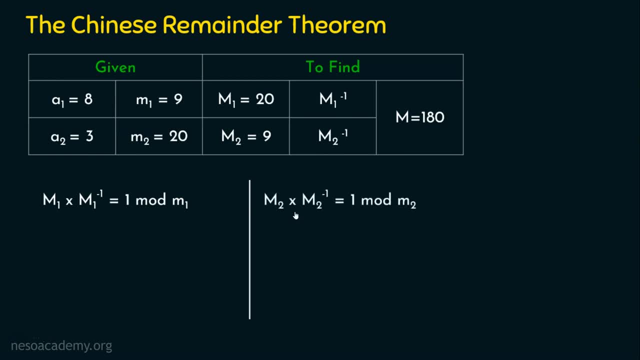 under mod small m1.. Similarly, capital m2, when it is multiplied by capital m2 inverse, we get 1 mod small m2.. We know what is the value of capital m1 and capital m2.. So firstly, let's focus on this equation. We get 20 into capital m1. inverse is equal to 1 mod. 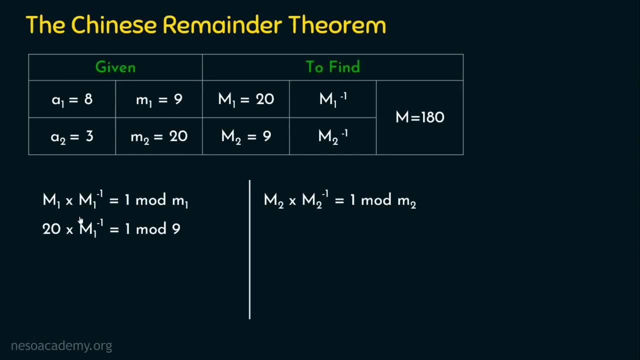 9, because small m1 is 9, which is this. So 20 into what we get the whole product. When it is divided by 9, we get 1 as the remainder. Let's start applying with 1.. You can also go for extended. 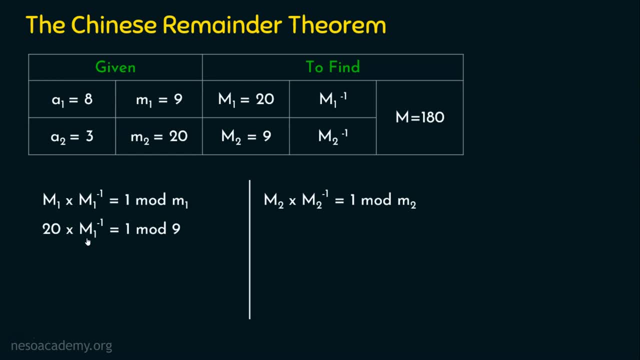 Euclidean algorithm to find the multiplicative inverse. Since these are all smaller numbers, I am going directly. Let's try with 1.. 20 into 1 is 20.. 20, when it is divided by 9, we get 2, as. 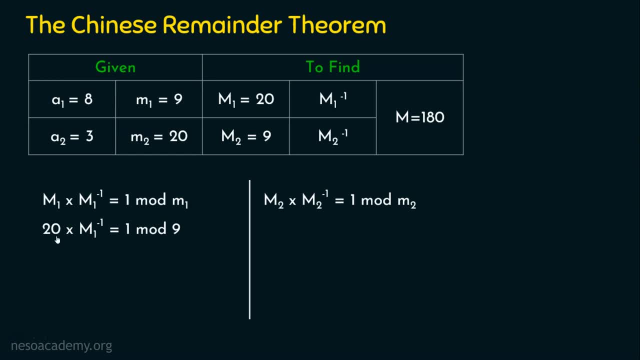 the remainder. So 1 is not the multiplicative inverse of 20 mod 9.. Let's try 2.. 20 into 2 is 40,. no, we don't get 1 as the remainder when we divide 40 by 9.. Let's try 3.. No, Let's try 4. No. 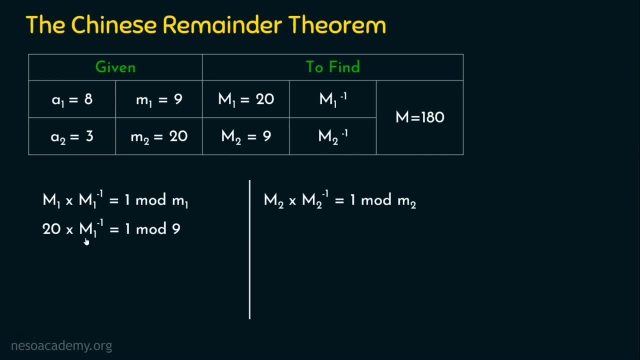 Let's try 5.. Yes, 20 into 5 is 100.. 100, when it is divided by 9.. 9, 11 times 99.. So we get 1 as the remainder. So obviously, capital m1 inverse is 5.. That's what we obtained. Let's move on to. 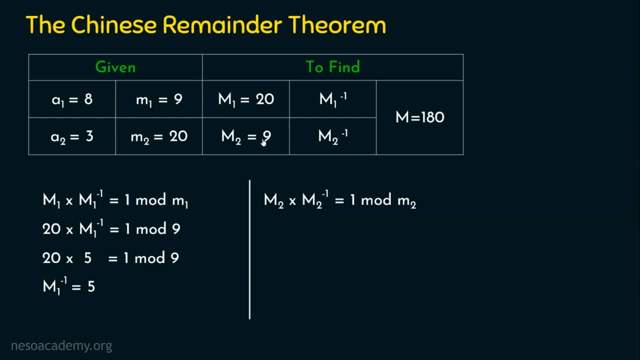 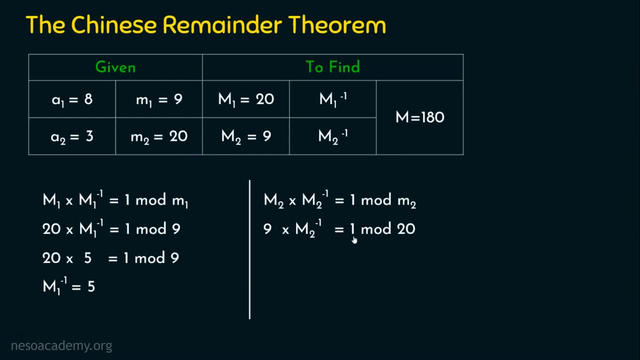 which is 20 here. So 9 into what we will get, 1 as the remainder when it is divided by 20.. So let's try with 1. No 2., No 3., No 4., No 5., No 6., No 7., No 8., No 9.. 9 into 9 is 81.. 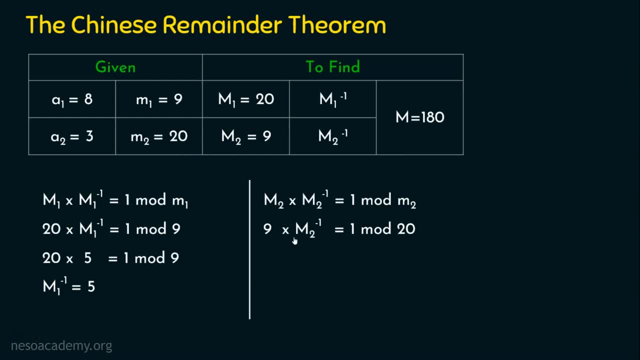 And we know what is small m2,, which is 20 here. So 9 into what we will get, 1 as the remainder when it is divided by 20.. So let's try with 1. No 2., No 3., No 4., No 5., No 6., No 7., No 8.. 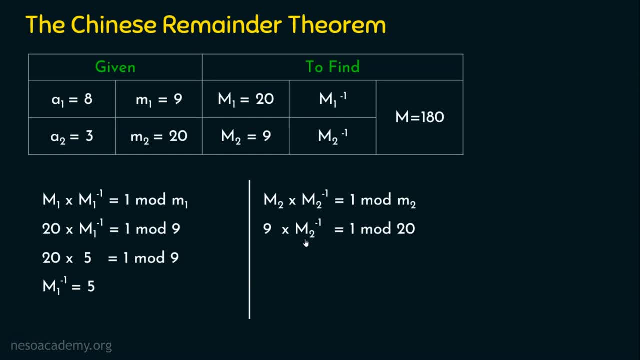 No 9.. 9 into 9 is 81.. 81 when it is divided by 20.. 24 times 80, we get the remainder 1.. So capital m2 inverse is 9.. We found out the value of capital m1 inverse and capital m2 inverse. 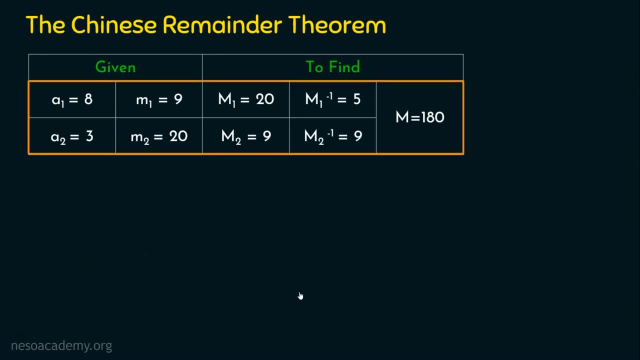 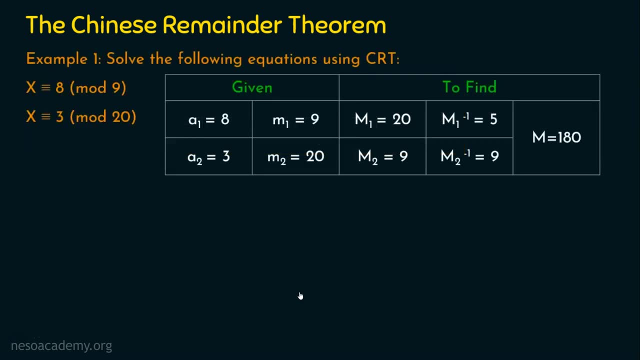 Let's place the values in the table. So we have found out all the values that are required to solve this problem. So let's take this value and place it here. Let's take the question. You can take either the original question or the rewritten question. Anyway, the final answer. 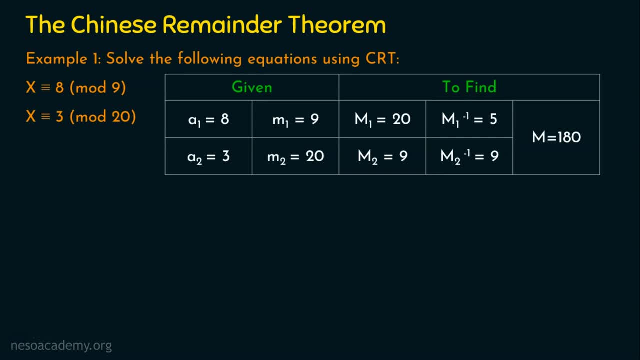 remains the same Here, I will take the rewritten question. So we are required to find: x is 8 mod 9 and x is congruent to 3 mod 20.. And we know the value for x can be obtained using this: 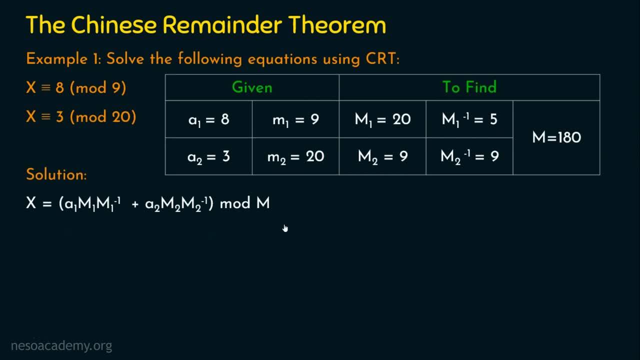 formula. We have all the required values on the table. So when we substitute the values, when we evaluate this expression, we get 1043 mod 180.. Why 180? Because this is mod m, which is 180.. So when we evaluate this, we get 143 as the value of x. It means 1043 when it is divided by 180,. 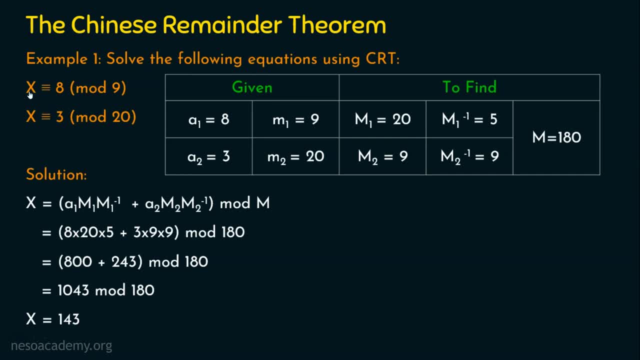 we get 143.. In 143, when it is divided by 9, we get 8 as the remainder. And 143, when it is divided by 20, we get 3 as the remainder. So we have verified the final result also. So we have found out x. 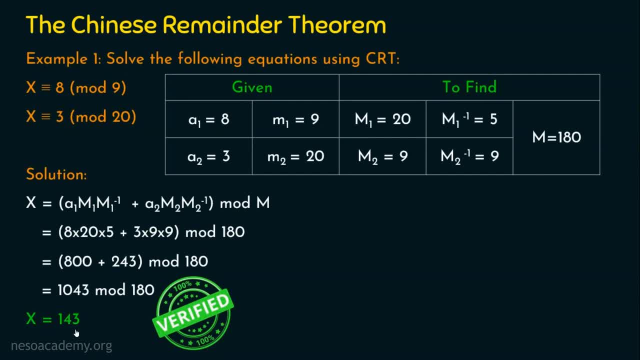 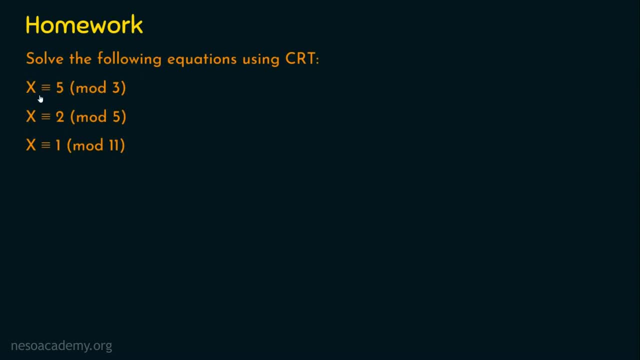 is equal to 143.. Before we sign out, let's see the homework question. The question is: solve the following equations using CRT. The equations are: x is congruent to 5 mod 3,, x is congruent to 2 mod 5, and x is congruent to 5 mod 3.. So we have: x is congruent to 5 mod 3,. 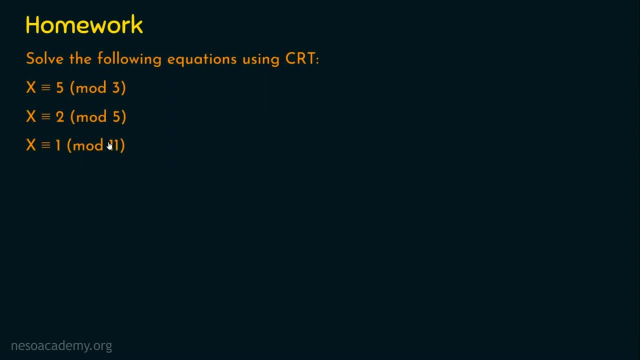 x is congruent to 2 mod 5, and x is congruent to 2 mod 5.. So we have: x is congruent to 5 mod 3, and x is congruent to 1 mod 11.. Please note here: 3,, 5, 11 are relatively prime to each other. 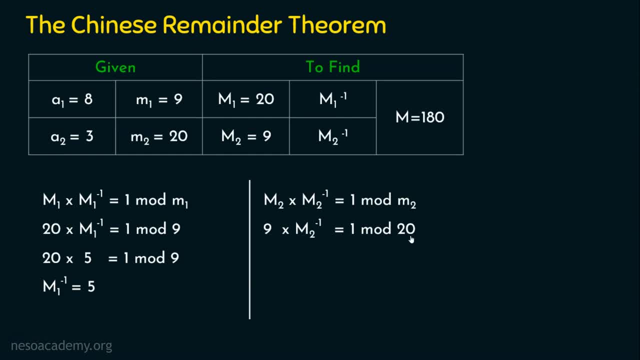 81 when it is divided by 20.. 24 times 80, we get the remainder 1.. So capital m2 inverse is 9.. We found out the value of capital m1 inverse and capital m2 inverse. Let's place the values in the table. So we have found out all the values that are required to 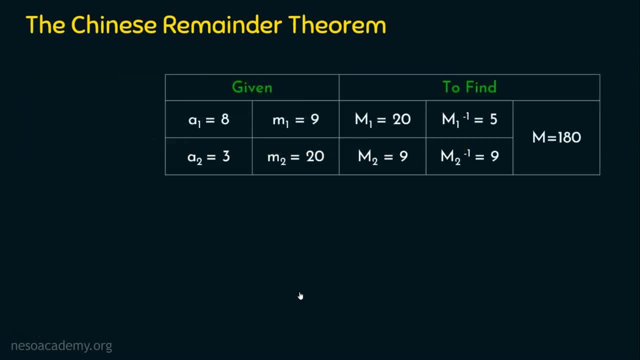 solve this problem. So let's take this value and place it here. Let's take the question. You can take either the original question or the rewritten question. Anyway, the final answer remains the same. Here I will take the rewritten question. So we are required to find x's congruent. 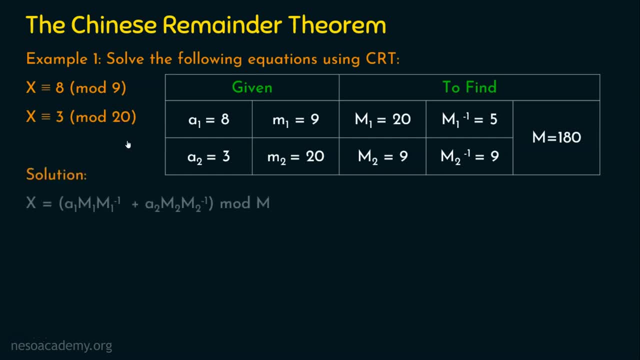 to 8 mod 9 and x is congruent to 3 mod 20, and we know the value for x can be obtained using this formula. We have all the required values on the table. So when we substitute the values, when we 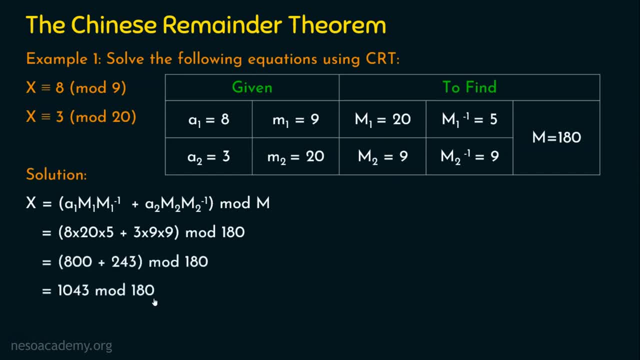 evaluate this expression, we get 1043 mod 180.. Why 180? Because this is mod m, which is 180. So when we evaluate this, we get 143 as the value of x. It means 1043. when it is divided by 180, we get 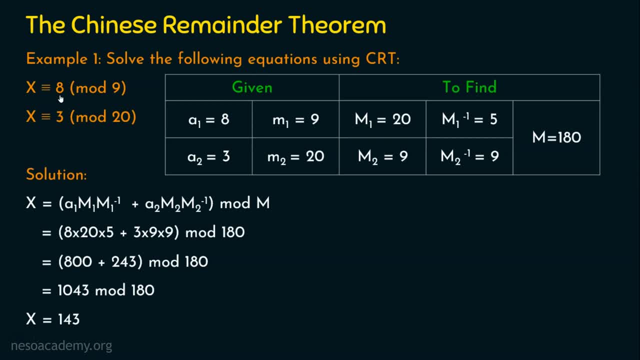 something like this: When 143, when it is divided by 9, we get 8 as the remainder, and 143, when it is divided by 20, we get 3 as the remainder. So we have verified the final result also. So we 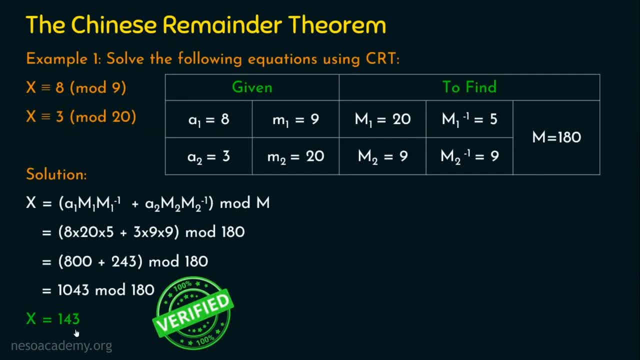 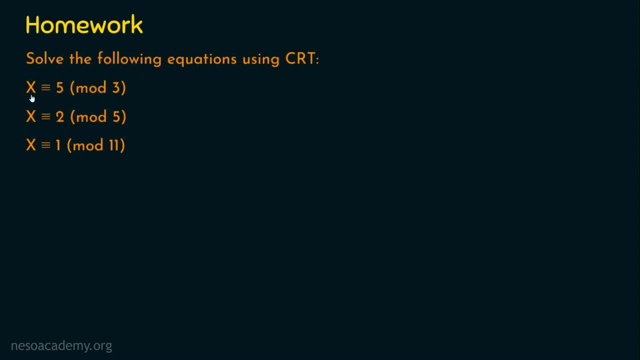 have found out, x is equal to 143.. Before we sign out, let's see the homework question. The question is: solve the following equations using CRT. The equations are: x is congruent to 5 mod 3,. x is congruent to 2 mod 5.. 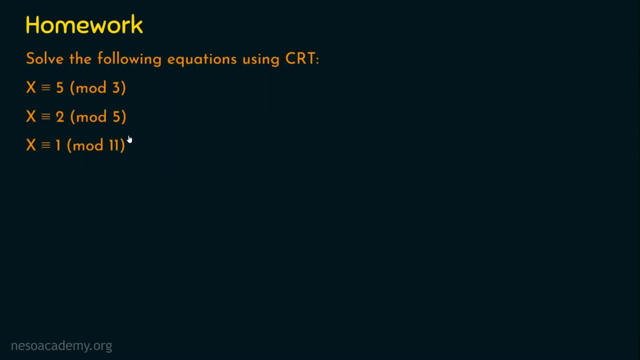 congruent to 1 mod 11.. Please note here: 3,, 5,, 11 are relatively prime to each other, Hence there exists a unique solution for this question. I request you to solve this question and post your answers in the comment section. 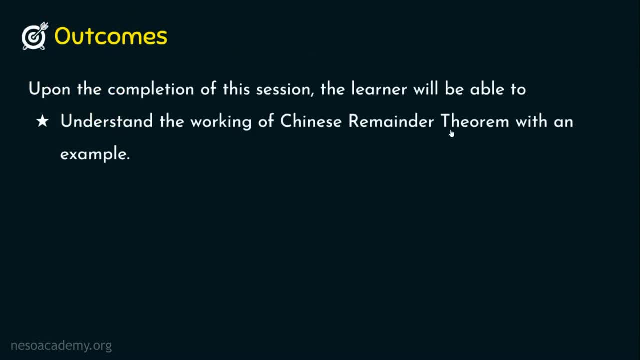 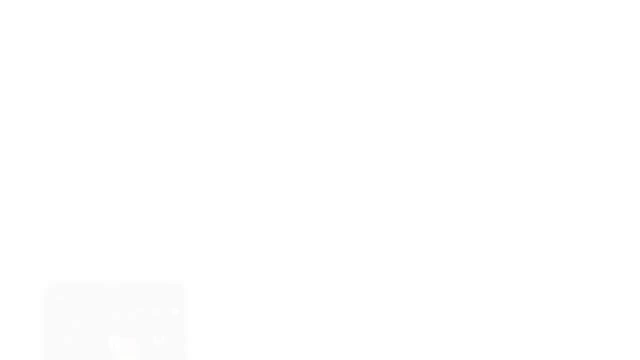 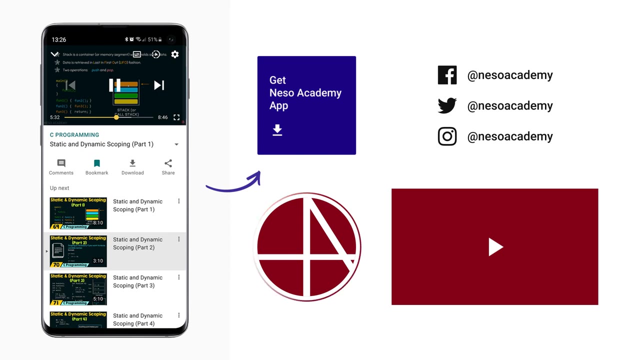 And that's it, guys. I hope now you understood the working of Chinese remainder theorem with an example. I'll see you in the next presentation and thank you for watching.